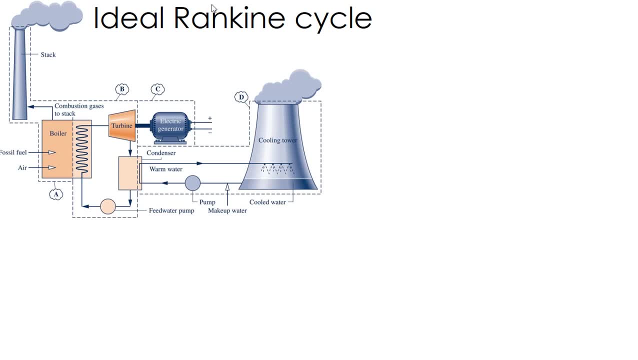 Based on environmental codes and things of that nature. Okay, but really we're going to focus on B in here And that's really the Rankin cycle. So combustion is outside the scope of this course. It's towards the end of the book, If you want to look at that. the electrical generator that's, you know, kind of outside of thermal altogether, taking rotational energy, turning into electrical energy, And we'll talk a little bit about the condenser, the cooling water, but maybe not necessarily the heat transfer that goes behind it. 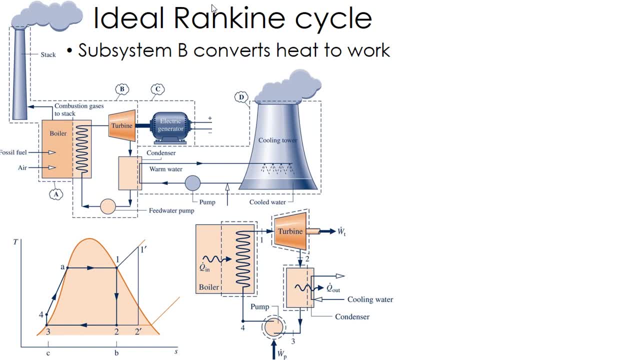 But the you know temperature, the cooling water coming in and out, Okay, but really the focus boils down to what's in B, which is our Rankin cycle. So I've got the schematic here. I've also got the temperature versus entropy diagram to help us go through things. Okay, And again, with our systems we go through and we go state by state, setting the state here, because I've got the fluid flow, I'm looking for H values. So once I get those H values, I can then 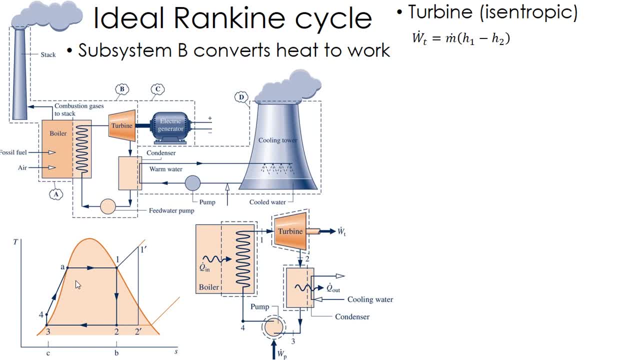 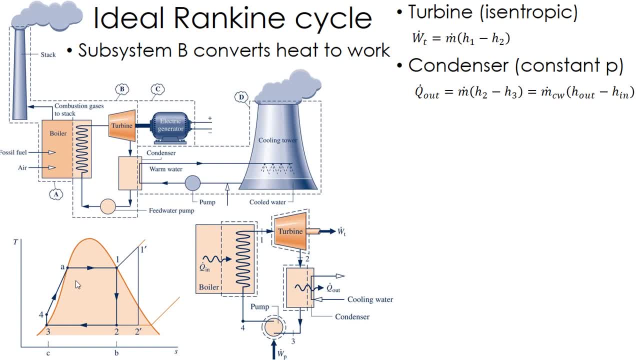 know two to three. okay, but we can also use that to help me again find what's going on with the cooling water. okay, where i've got a different mass flow of cooling water, uh, in and out, i can use those h values you know. that'll help me find. uh. it could help me find the mass flow rates, could. 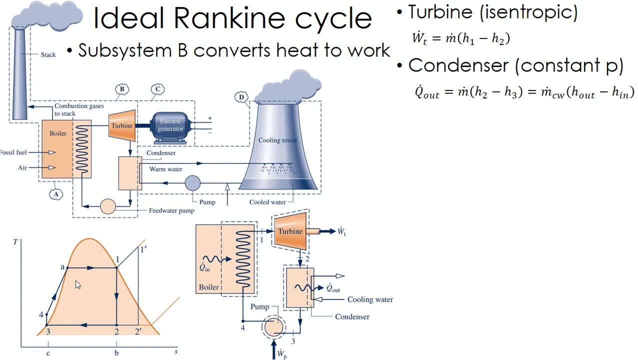 help me find temperatures in and out of the cooling water, different things of that nature. again, that cooling water is separate process one, two, three, four is really what we're looking at. okay, the pump is also isentropic. now, if you'll remember, we talked about an isentropic steady state flow of an incompressible. 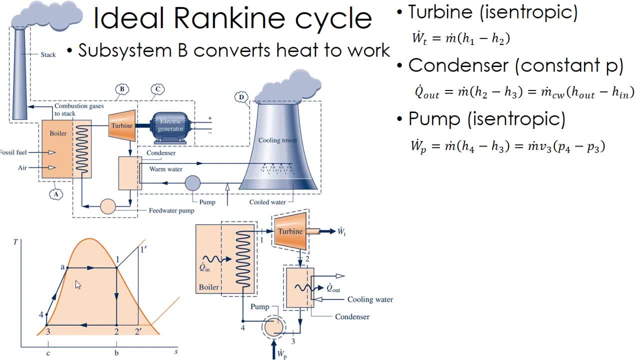 fluid, okay, so really, my, i mean we already know that it's delta h, right, but it's also v, delta p, if you look back into the last section of chapter six. okay, and we're going to use that to our advantage, because oftentimes we know that it's a delta p and we're going to use that to. 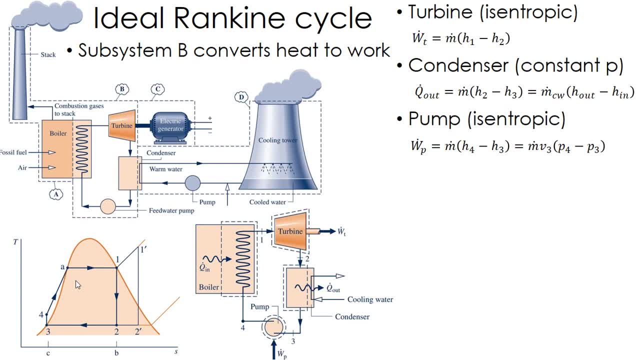 advantage because oftentimes we know that it's a delta p and we're going to use that to our, our pressures. we can actually use this V Delta P to help me set that final state H, because again, those H values are what is completely crucial to us and keep in. 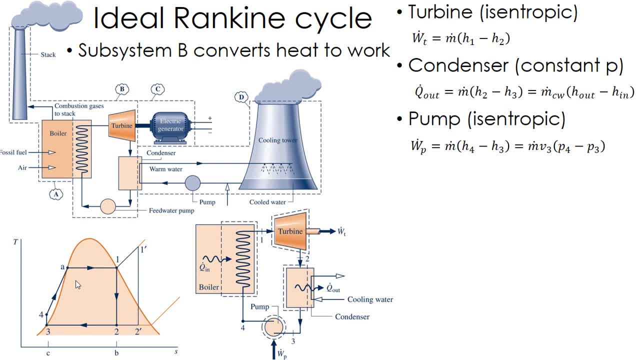 mind. with the pump we're in liquid, so a lot of times we don't have tables, so we use the pressure to help me figure out that, that H value that I'm looking at, okay, and then the boiler. again, there is a constant pressure. there's no work. 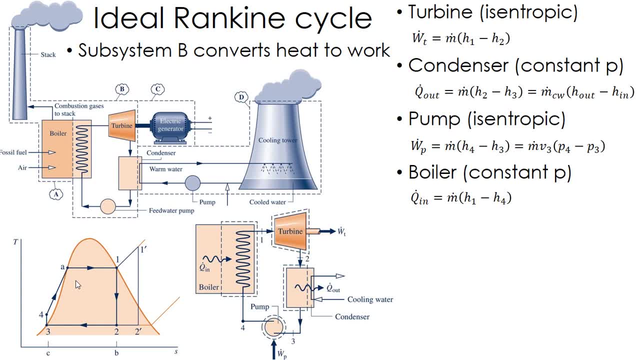 being done. so really, the Q in is just Delta H. one thing to keep in mind: these have directions. right, we talked about directions when we talked about entropy. okay, so we're always getting positive values here, but again remember, Q out is negative. you know, in the general sense of a first law, right work out is 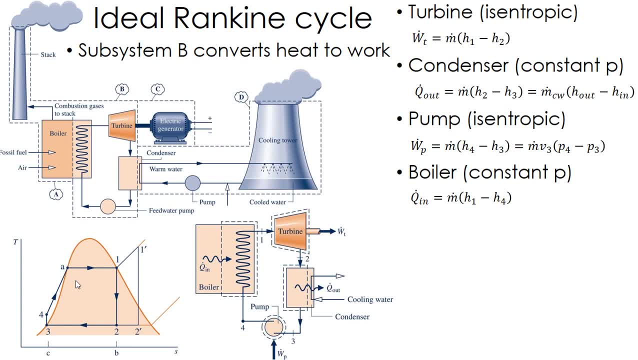 positive, okay. but again, these are giving me the direction. you can see, the work of the turbine is out, the work of the pump is in, so the turbine is positive work out. the pump is out is positive, work in, okay. but again, when we apply that first law, just remember: 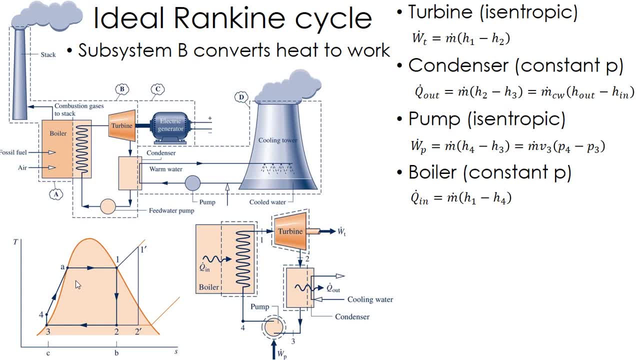 how things are going. we like positive numbers, but these have directions, okay. so when we get to our thermal efficiency, the work of the cycle is the work of the turbine minus the work of the pump- okay. or the positive work of the term: turbine minus the positive work of the pump- right. the pump is, there's work being put. 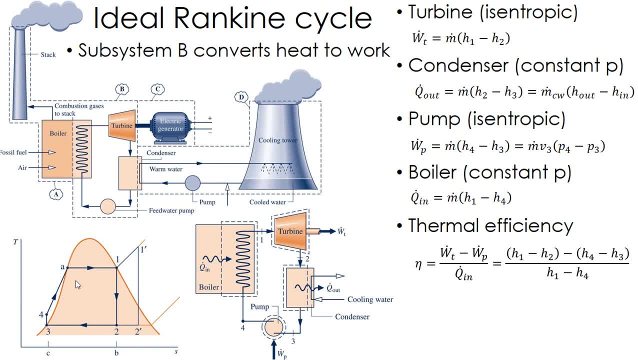 onto the system, so it's negative work and then we simply have to draw back. the turbine is out. that's where that negative sign comes from. but all of these values, again, we generally deal with in positive terms: knowing the direction, whether it's in or out, that sort of thing. 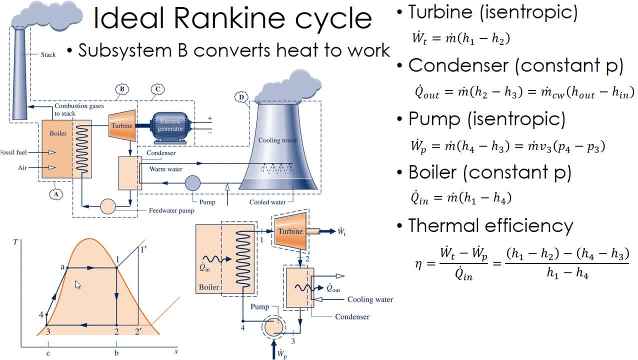 okay, so again it's the work of the cycle over q in, where q in again is the, the, the q of the boiler. okay, then we have a back work ratio. that's really just the ratio of the pump to the turbine. okay, and generally we want this low, we want to get more out than what we're putting in, sort of thing. so 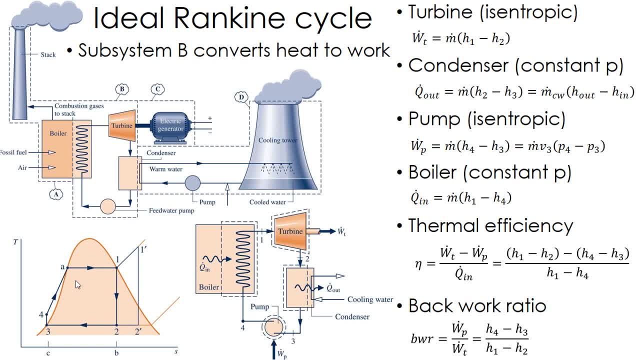 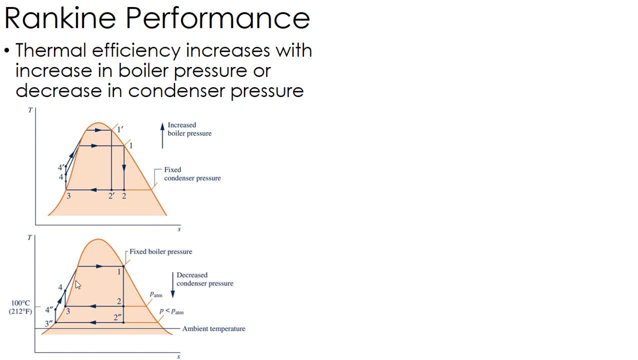 as low as possible is generally good. it's just a value that sometimes useful to to have. okay now, as far as performance of this rank and cycle, okay, you remember when we talked about the carno cycle? right, the bigger the difference in the temperature, better performance. whole idea, same thing happens. 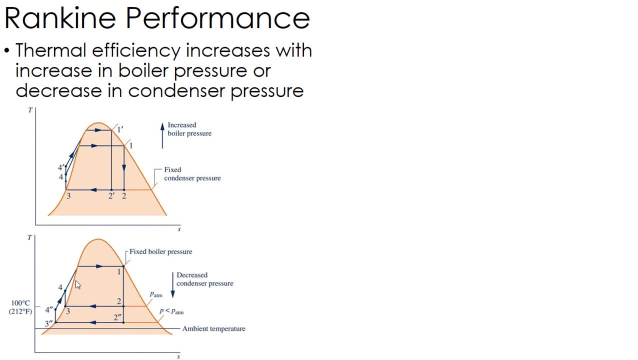 here. right, if i increase the pressures, that's going to result in the temperature going up. right, increased pressure under the vapor dome means increased temperature. okay, so again, when i have that bigger temperature difference or that bigger pressure difference in a case here, my thermal efficiency is actually going to be better. now I have some limits here. for example, you can't: 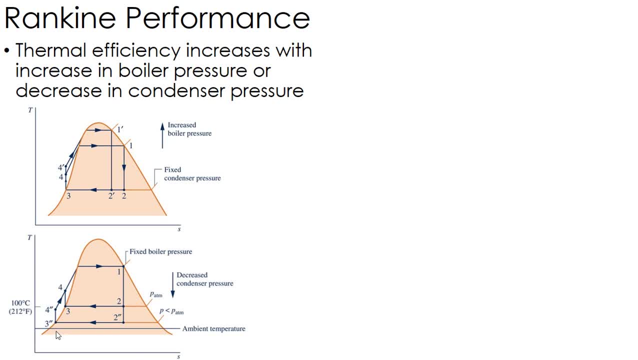 the lower pressure. you don't go below. you know the ambient temperature, because otherwise you won't get the heat out that you need. so you're kind of limited by whatever the ambient temperature is for how far down you can take the the low pressure. okay, because you still need that heat. 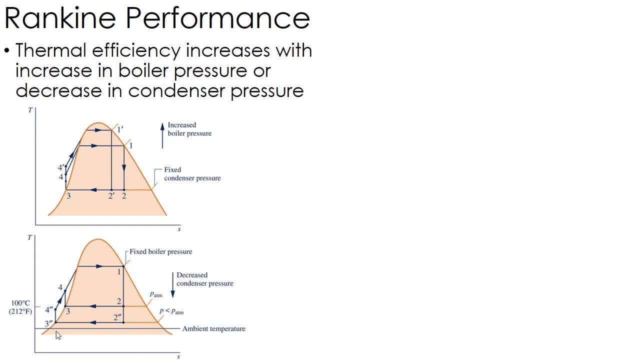 transfer going from a hotter to a colder sort of idea. okay, but in general, the bigger you push these pressures in both directions, the better your performance will be. now let's go ahead and compare this to the Carnot cycle, right? so the Carnot cycle is the rectangle right where we've 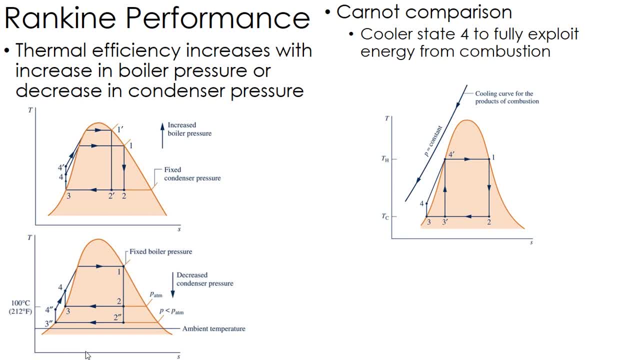 got isothermal, isentropic, back and forth. okay. so the thing here is to to exploit what's going on with combustion, which again we haven't got. you know that's beyond the scope of the course that we're dealing with here, but generally we want as cool of a temperature as 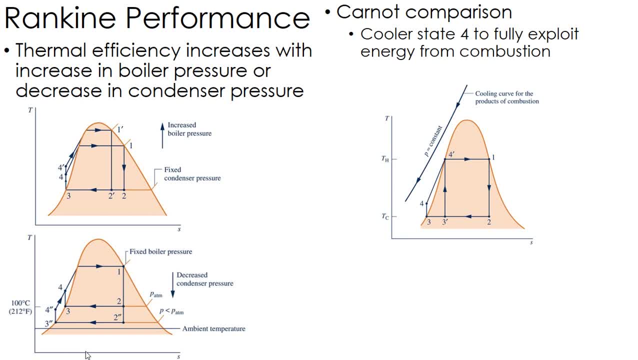 possible for state four going into the boiler so I can get that bigger temperature difference to get kind of a more efficient heat transfer again, kind of beyond what we're talking about in this course. but you get the idea that if I've got a lower temperature going into the boiler I'm going. 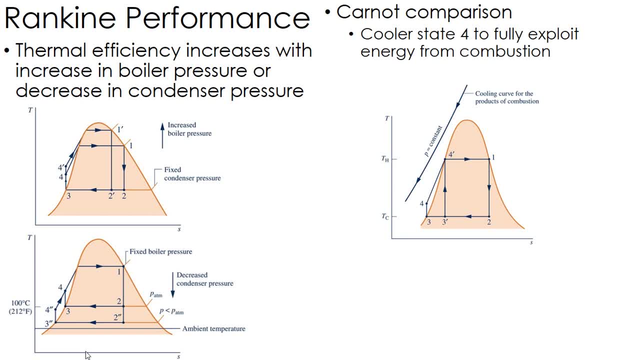 to get a lot more heat transfer from the combustion gases to the to the. you know the boiler stream that I've got going on here. okay, so that's one aspect. the other aspect is pump, which is process three to four. it can really only handle a single state, it can only handle a liquid, so we got to push three all the way down to the. 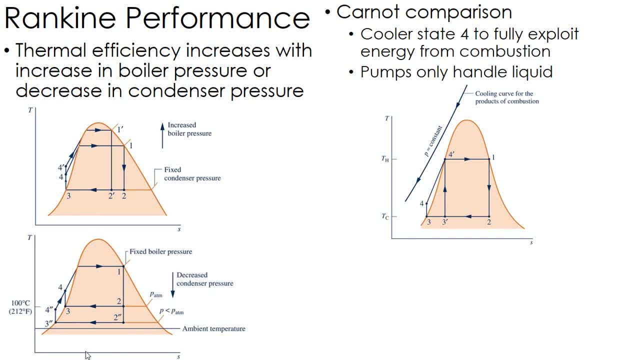 the saturated liquid, pump it up to a higher pressure, then throw it into the boiler. okay, because of that, though, I have a decreased performance compared to, again, the ideal situation, which is a Carnot cycle. okay, but in in actuality, you know, there's some limitations to that Carnot cycle, so we, we use this. 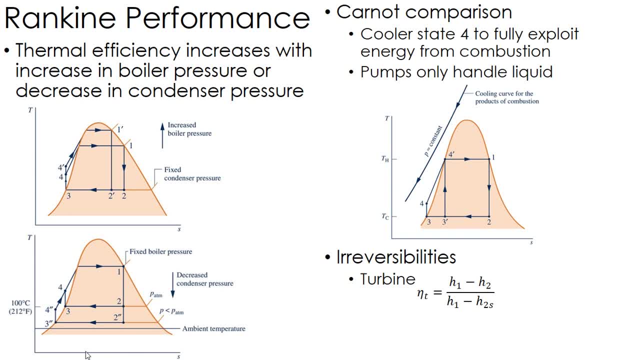 Rankin cycle. okay, now again, we could have some irreversibilities. keep those in mind. okay, in the previous slide we were talking about the ideal situation. you know I- here's a little bit of a plot here. I have a turbine. it could have a, an isentropic efficiency we talked about. okay, ideal would be. 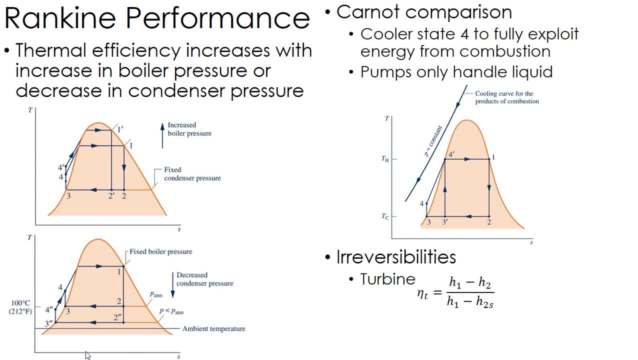 constant entropy- okay, then you know. so that's the h2s, I could find the best case. and enthalpy: okay, use that too. and then, knowing that I have a 90 percent efficient turbine, I can find the actual enthalpy at State two. again, the whole idea is setting these states. same thing happens with the pump. 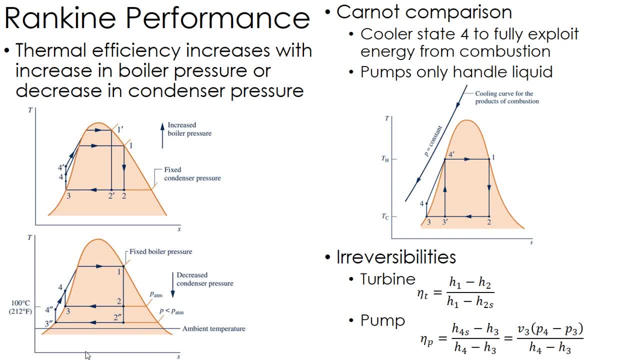 just kind of the reciprocal of that where it's the best case over the actual case. remember, the best case is also that isentropic steady state flow of an incompressible fluid, right where that's v delta p. so again we can use that v delta p to actually help us set state four. find that 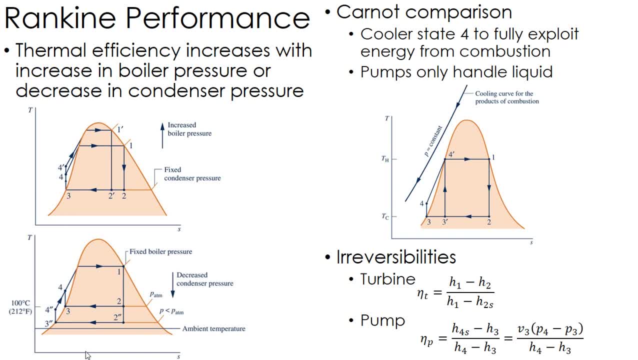 enthalpy of state four, which again is going to be necessary to find kind of q in and things of that nature to help us set our state okay. so you know, if you have efficiencies then you need to apply that again. we talked about that back in chapter six. so that's the the initial ideal uh rank and 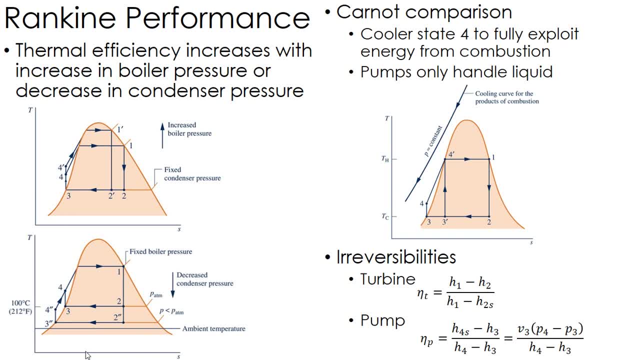 cycle. we'll add to this as we move along, but that gives you a handle of the the initial idea of it.